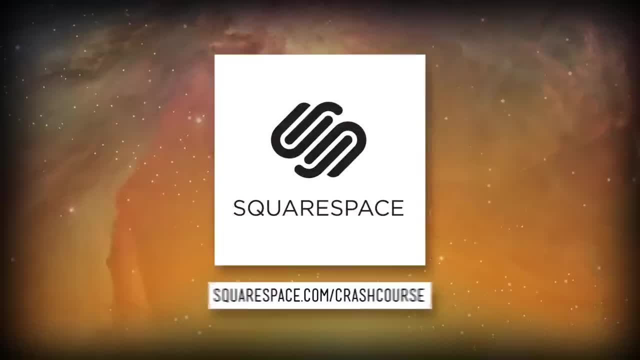 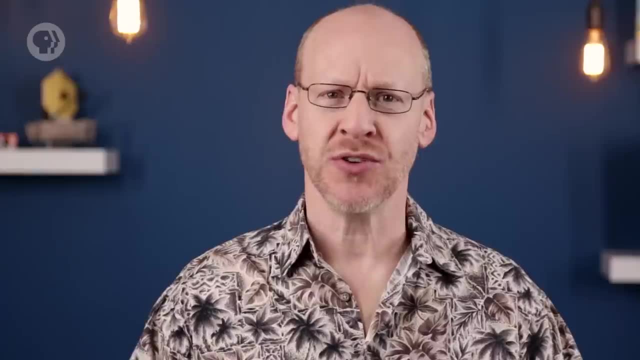 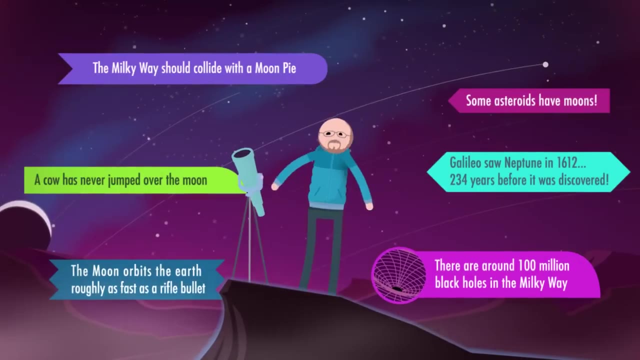 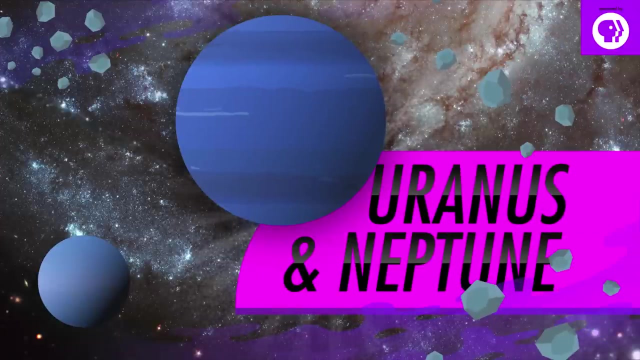 This episode of Crash Course is brought to you by Squarespace: Uranus, U-ran-us, U-ran-us, U-ran-us, U-ran-os. There are five planets in our solar system. you can see without a telescope, Well, six. 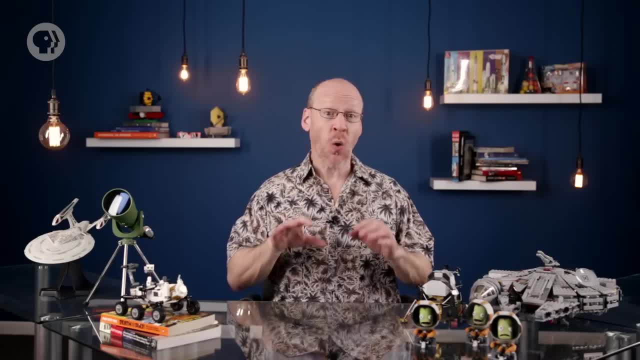 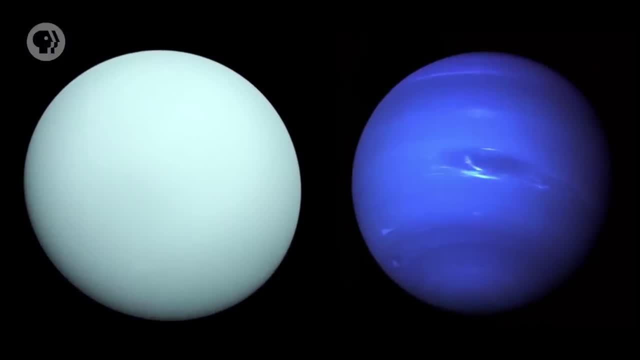 if you include the one you're sitting on, But there are two more big ones out there orbiting the Sun out in the cold depths of the outer solar system: Uranus and Neptune. They're a lot alike in many ways, but of course they have their individual quirks. 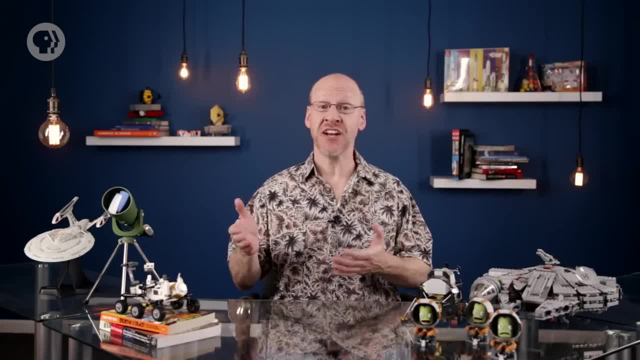 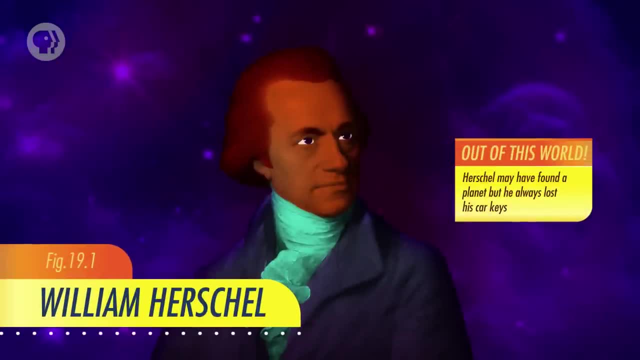 Uranus was the first planet to be discovered, and by that I mean it wasn't known in ancient times. It took an astronomer with a telescope to find it. In 1781, William Herschel was mapping the skies through his telescope when he spotted a greenish object. that was clearly 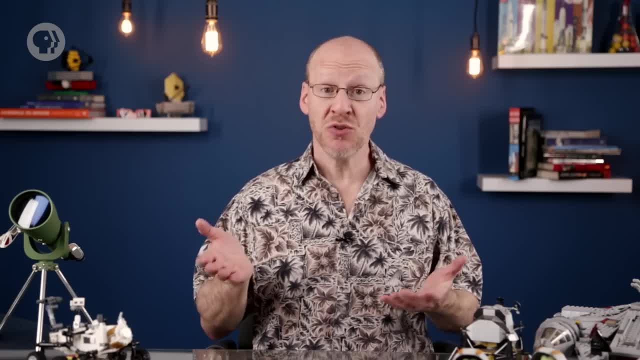 a disk and not a dot like a star. He noted its position and moved on. but when he went to observe it again, he found that it was not a dot like a star, It was more like a star. When he looked at it again sometime later, he was astonished to discover it had moved. 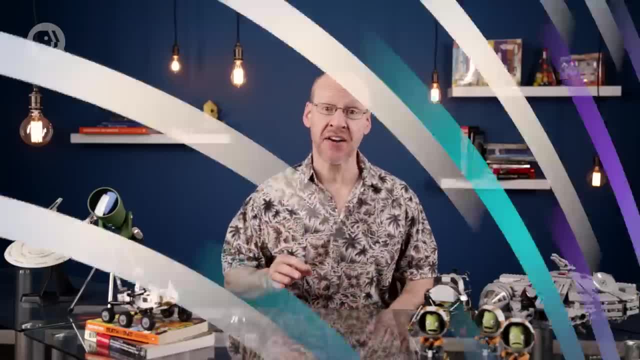 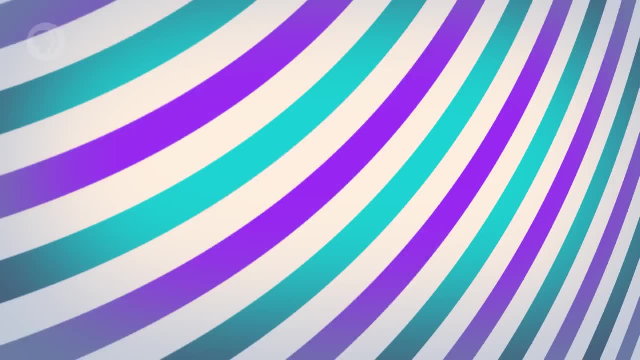 It was quickly determined to be a planet more distant from the Sun than Saturn. In true brown-nosing style, he named it Georgium Cetus, or George's Star, after the reigning king George III. Yeah, happily that name didn't stick and keeping with the nomenclature of 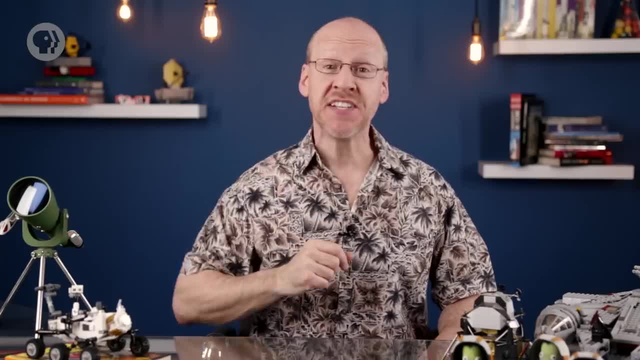 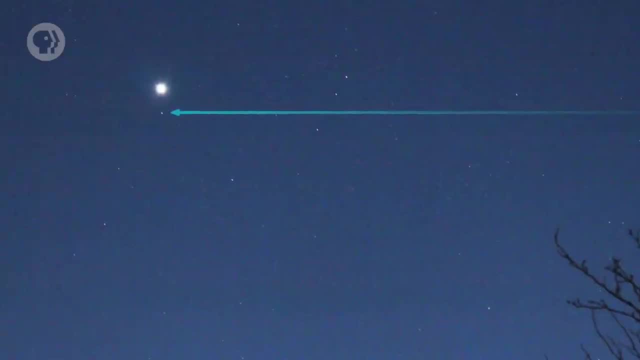 Roman gods, the new planet was dubbed Uranus. Interesting tidbit: It actually is visible to the unaided eye. if you have very sharp eyesight and very dark skies. It's right on the thin, hairy edge of visibility. What's funny is that several people had observed it before Herschel, but none had noticed its. 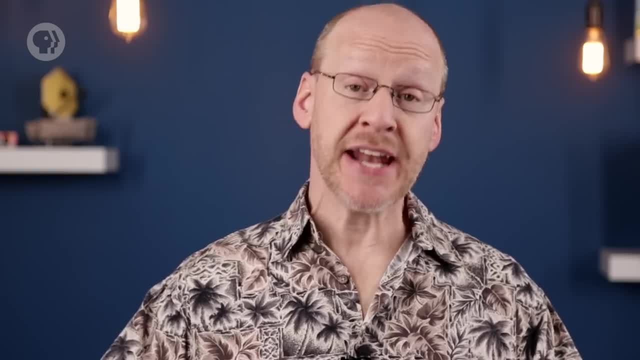 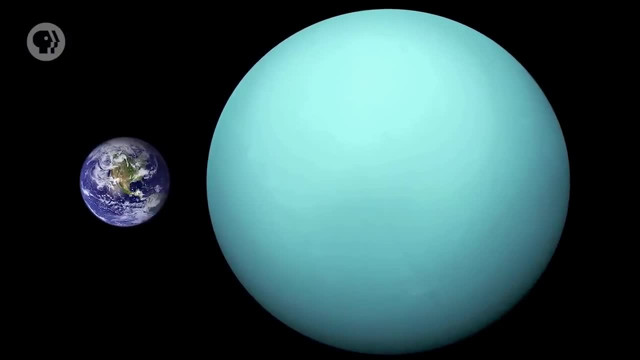 movement. Some even cataloged it on their maps as a star. The planet is massive, about 14.5 times the mass of Earth, but not terribly dense. This means its interior must be made of lightweight stuff, Scientific models of the planet based. 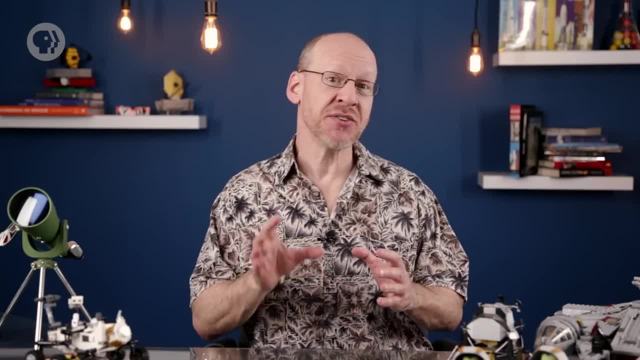 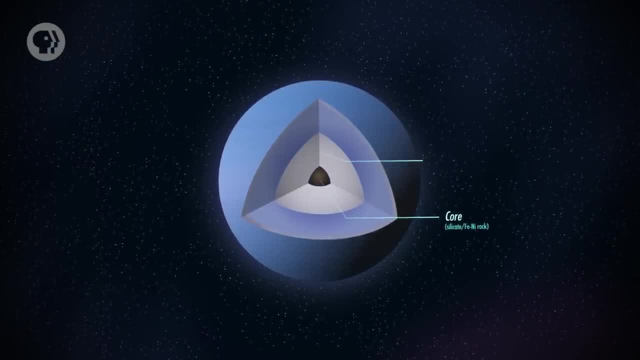 on physics and chemistry of the outer solar system indicate, its interior is probably made up of three general layers. There's a small rocky core, smaller than Earth, surrounded by a very thick layer of materials like water, ammonia and methane. This mantle makes up the bulk of the planet, in fact, and is dense, hot and under a lot. 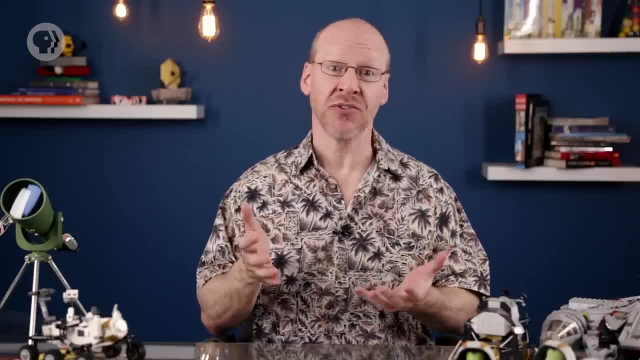 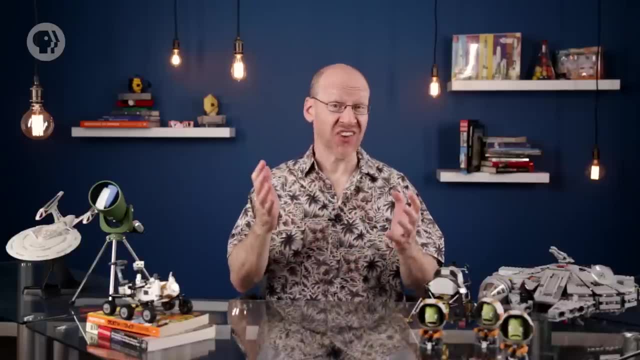 of pressure. In many ways, it's more like an ocean than anything else. However, somewhat confusingly, I'll admit- outer solar system planetary scientists refer to water, ammonia and methane as ice. So, even though it's not ice like we usually, 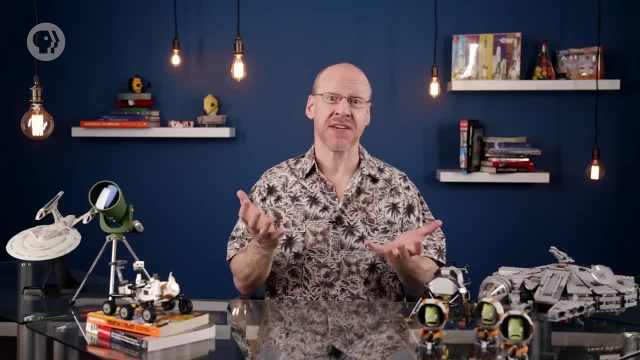 think of it. here on Earth, we say that the mantle of Uranus is icy. To distinguish it from the gas giants Jupiter and Saturn, Uranus is called an ice giant. Speaking of ice, here's a really weird thing. Studies have shown that the pressure of the 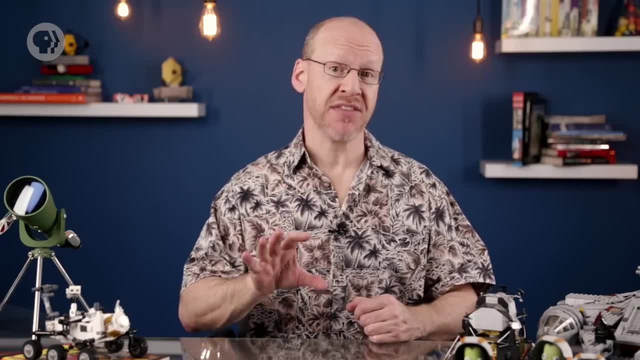 mantle of Uranus is the same as the pressure of the mantle of Saturn. The mantle of Saturn is the same as the mantle of Uranus. The mantle of Saturn is the same as the mantle of Saturn. The pressure inside Uranus can break up methane molecules, squeezing the carbon in them, so 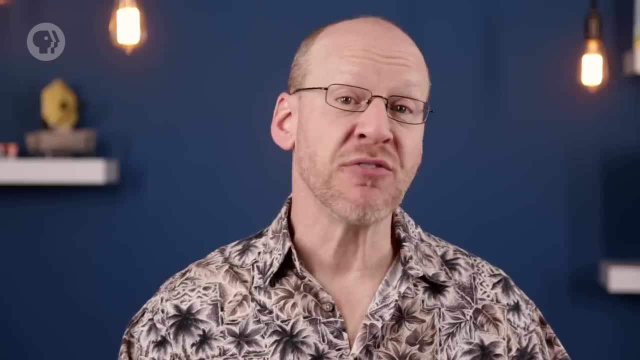 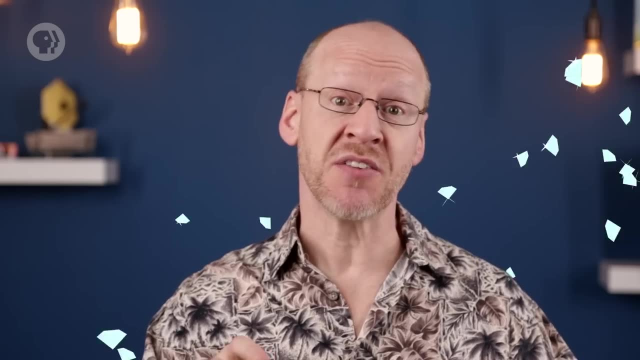 tightly that it actually forms diamonds. These would then fall down to the base of the mantle like sparkly hailstones. Except it's dark But still. down there in the depths of Uranus, there may even be an ocean of liquid diamonds, where solid ones float like diamondbergs. 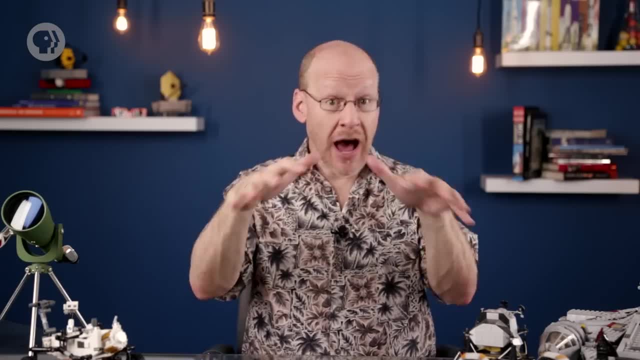 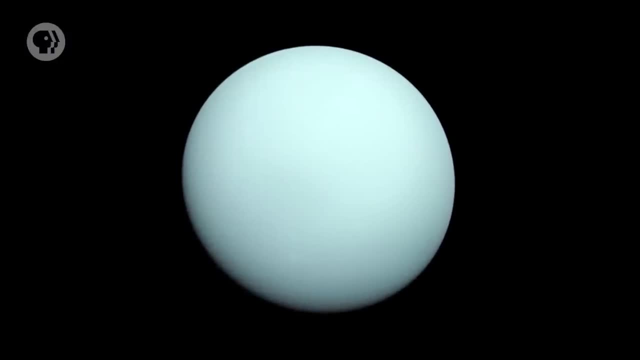 Not that we'll ever see that When we observe the planet, we're only seeing the top of its atmosphere. Besides hydrogen and helium, the air there is about 2% methane. Methane is really good at absorbing red light, which means the light we see reflected from Uranus. 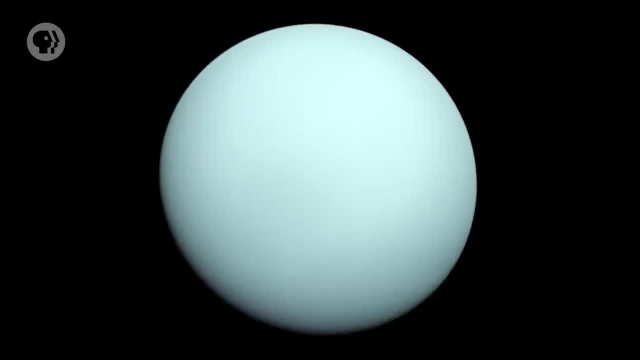 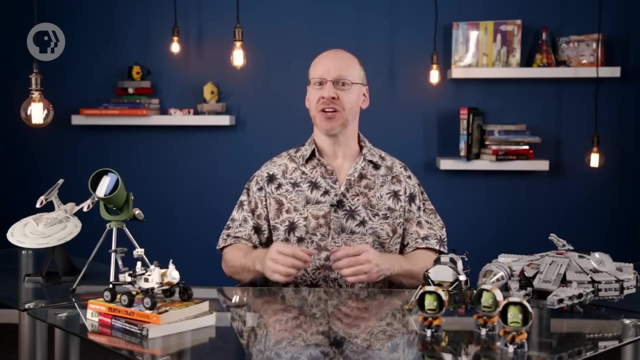 is mostly green and blue, making the planet look distinctly cyan or aquamarine, And it's pretty striking through a telescope, But in visible light the planet looks almost featureless. It doesn't have that deep banding like Jupiter or even the pale ones of Saturn, Though when 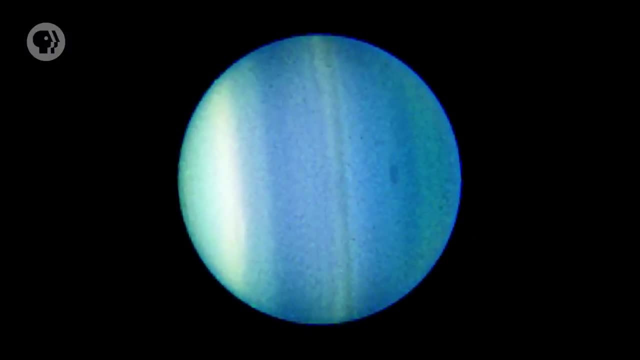 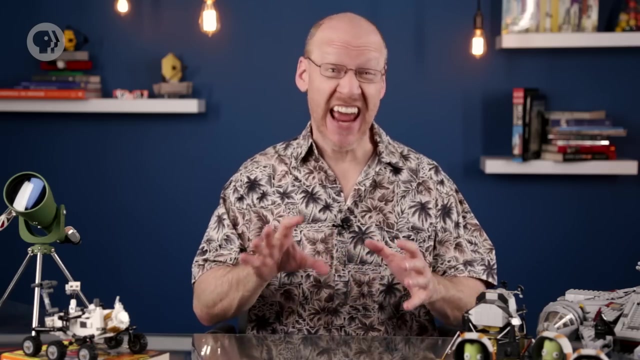 you look in the infrared, some banding can be seen. There are clouds, but again, they're difficult to see in visible light. The clouds are made of methane, ammonia and hydrogen sulfide. That last one is what makes rotten eggs smell so bad. I'd avoid breathing through your nose at Uranus. But then the atmosphere there is about negative 220 degrees Celsius, so that might be a better reason not to inhale. In late 2014,, a bunch of storms popped up in Uranus's atmosphere. 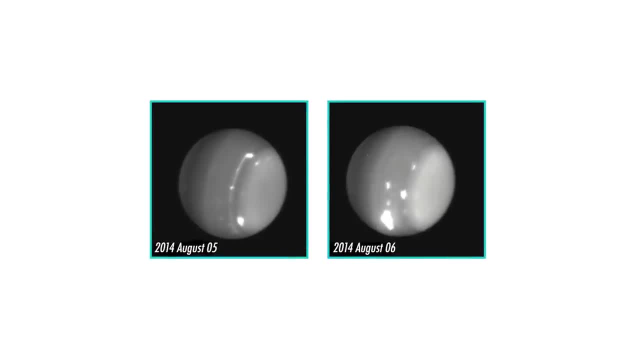 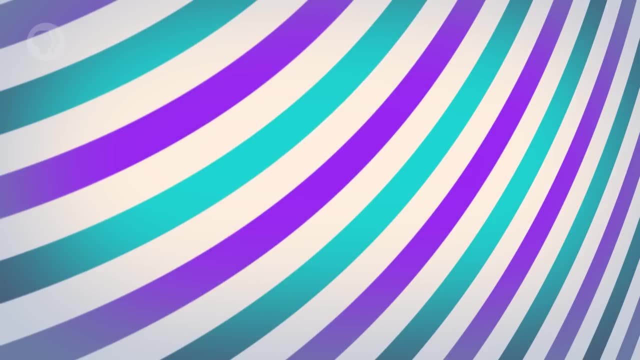 so big and bright they were easily visible from Earth. The storms may have dredged up very reflective methane ice from lower down in the atmosphere, and this time I do mean icy ice, which is why they were bright. The northern hemisphere of Uranus is approaching. 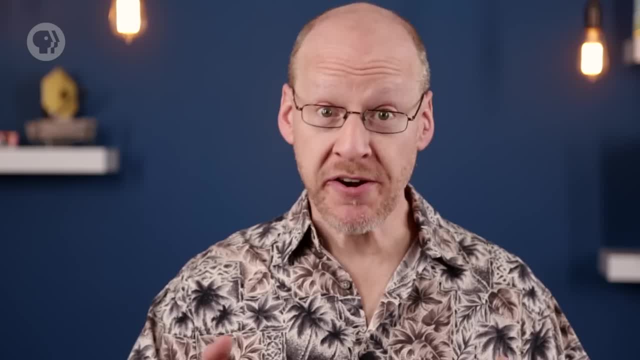 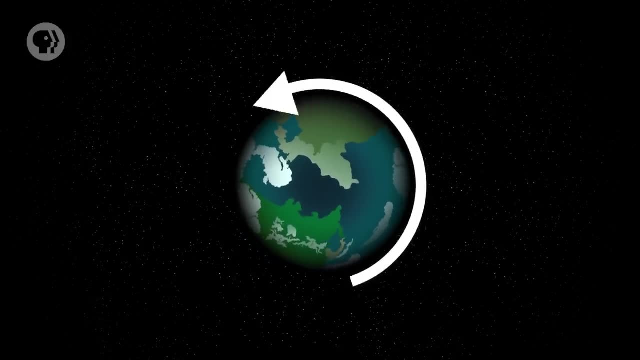 summertime, which may be why these storms formed. And that brings us to the weirdest thing about this planet: It's sideways. If you were above the Earth's north pole, looking down, you'd see our planet spinning counterclockwise west to east. The Sun spins. 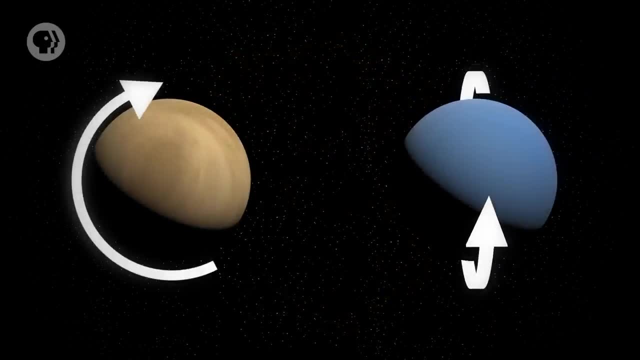 that way, and all the planets do as well, Except Venus and Uranus. While Venus is flipped all the way over, Uranus is tilted by about 98 degrees. That means that in the summer its axis is pointed almost directly at the Sun. so seasons on Uranus. 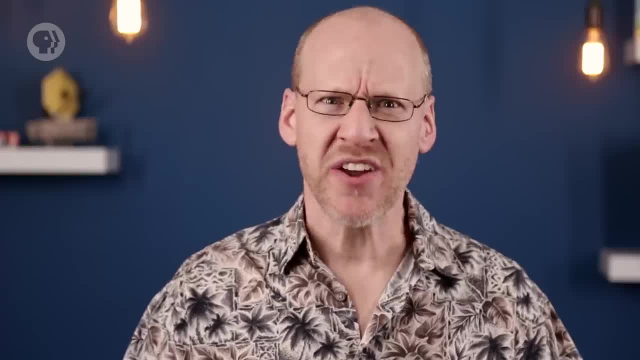 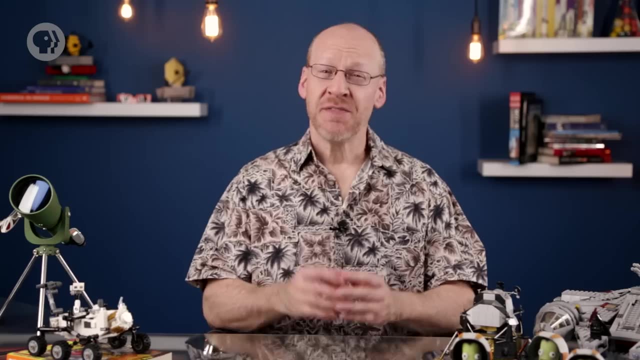 are pretty extreme by outer solar system standards. Weird. No one knows why Uranus is tipped so much. An obvious thought is that it got whacked hard by an impact long ago. If it were a grazing collision by a big object, that could have pushed hard enough on the planet to tip it. 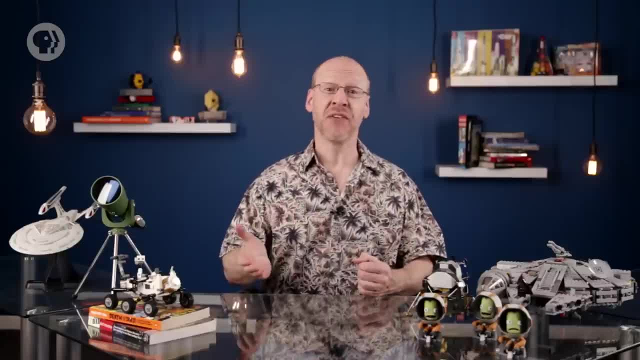 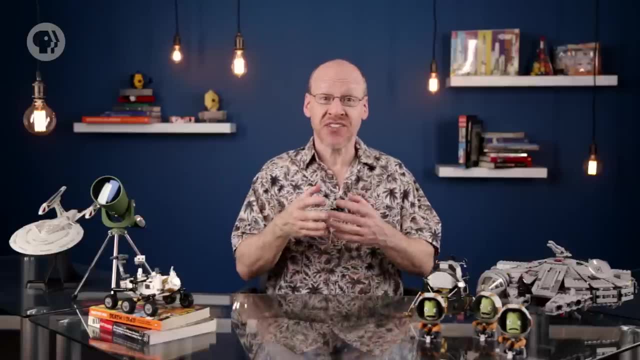 over. Unfortunately, Uranus is very far away and has only been visited by spacecraft once- Voyager 2 in 1986. And even then it was a quick flyby. Uranus's weird tilt is just one of those many mysteries that astronomers are trying. 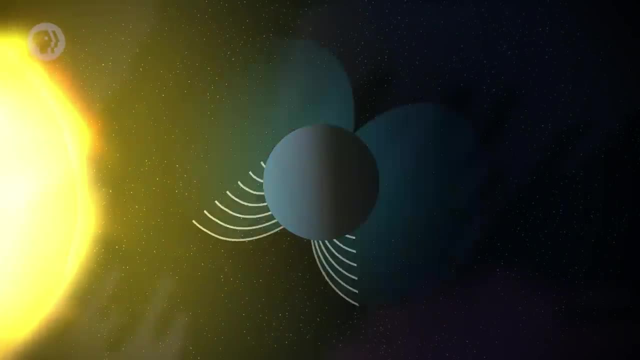 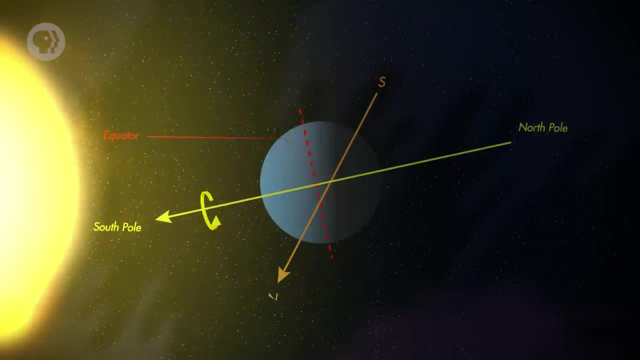 to solve with limited data. Uranus has a magnetic field, but it's truly odd. Its axis is tipped over by 50 degrees from the planet's spin axis and it's way off-center. The center of the magnetosphere is about 8,000 kilometers from the planet's center. 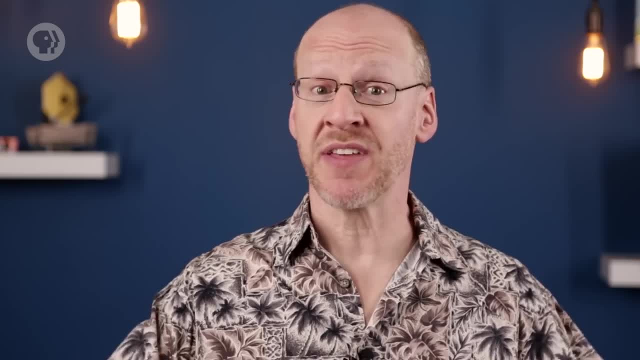 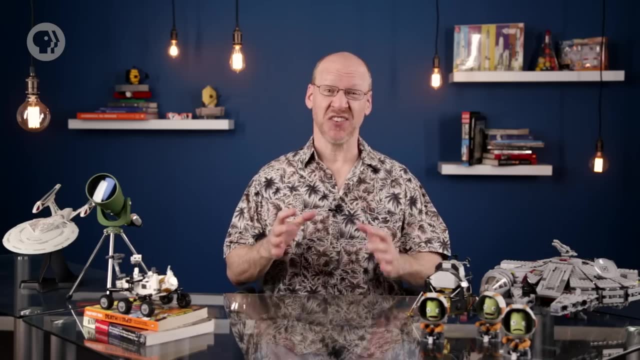 It may be that the magnetic field is generated in the icy mantle or that the core somehow interferes with the magnetic field, throwing it off. Truthfully, no one really knows why Uranus has more than two dozen moons, five big ones and a bunch of dinkier ones Cool. 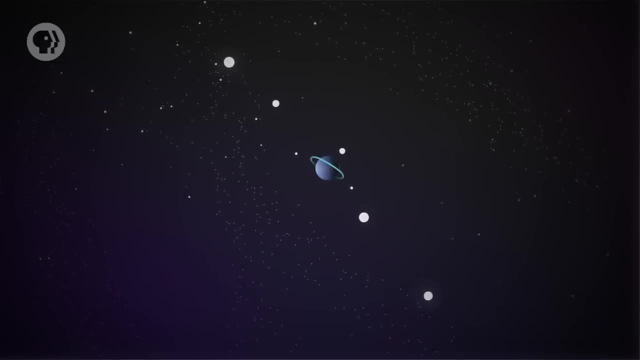 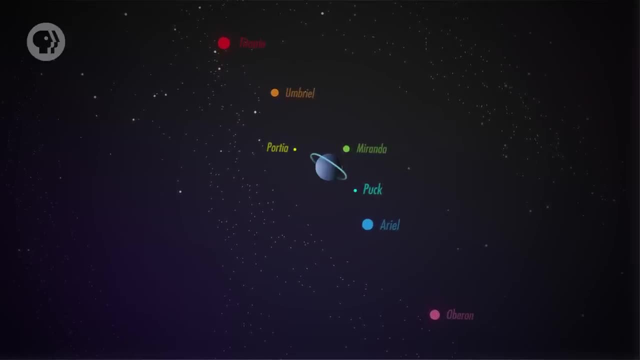 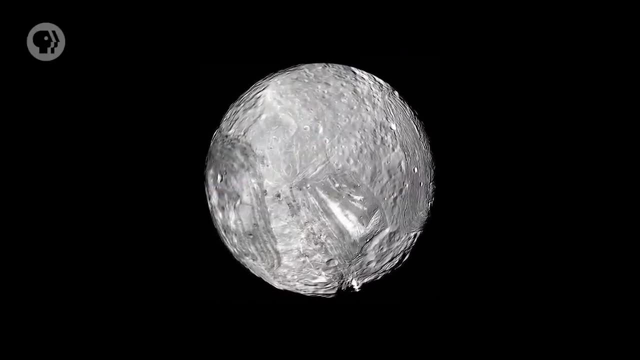 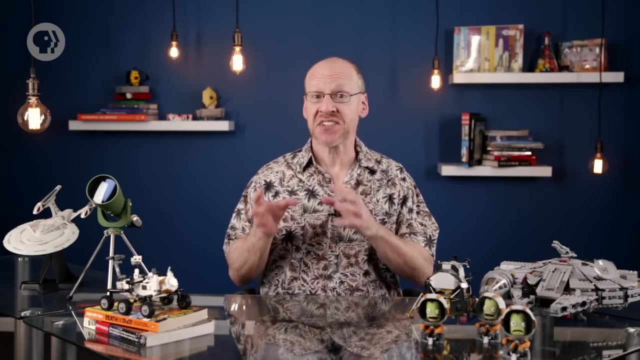 icy world that looks like it was put together by Doctor Frankenstein: A patchwork of jumbled terrains, all crammed together, crisscrossed by canyons and grooves. It's possible a giant impact in its past actually disrupted the Moon somewhat and it settled together. 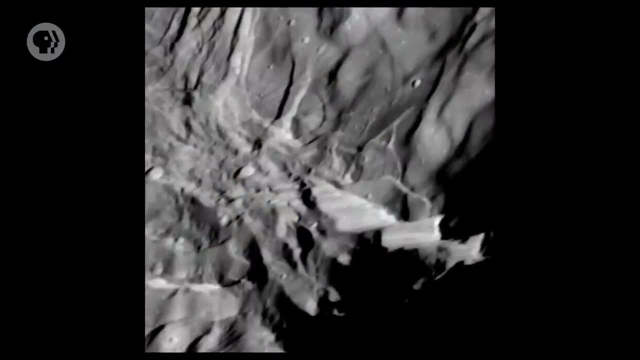 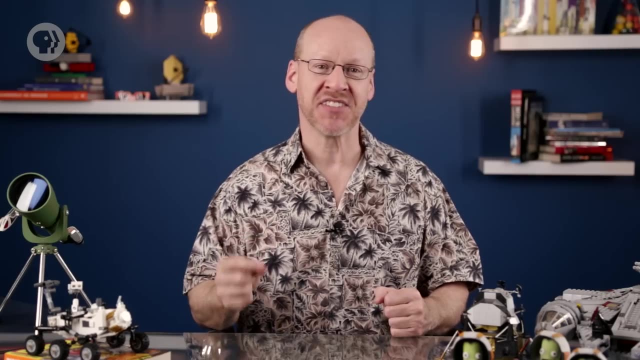 into this weird mish-mash, But the reason I like it so much is features called Verona Rupees. It's the tallest cliff in the Solar System, 5-10 kilometers high If you're. If you jumped off the top, it would take you six minutes to fall to the surface. 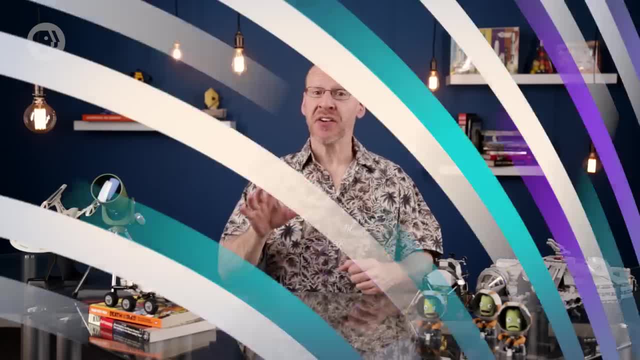 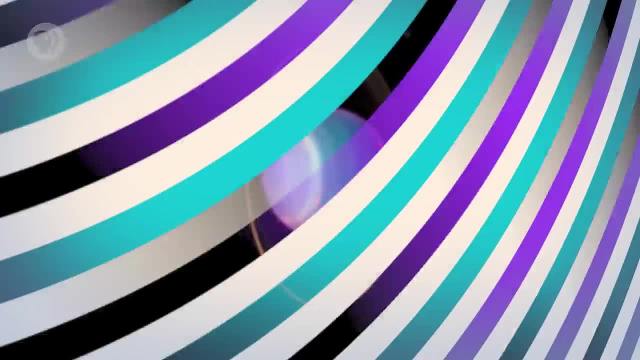 That would be a fantastic ride. Like Jupiter and Saturn, Uranus has a ring system too. They were discovered by accident in 1997.. Astronomers were observing Uranus pass directly in front of a star. They were hoping to use this to gather information about the planet's atmosphere as starlight. 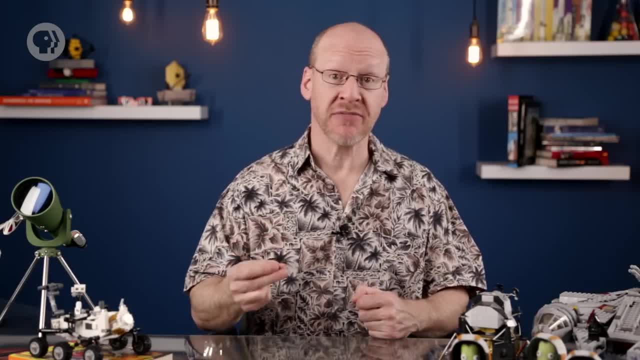 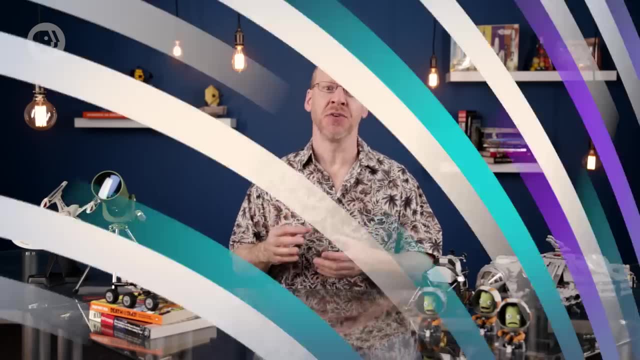 passed through it, But they saw several dips in starlight before the main event, which they realized were from rings around the planet. The rings are made of dark particles, probably ice, and reddish organic molecules. There are 13 rings known. most of them are very faint and narrow. 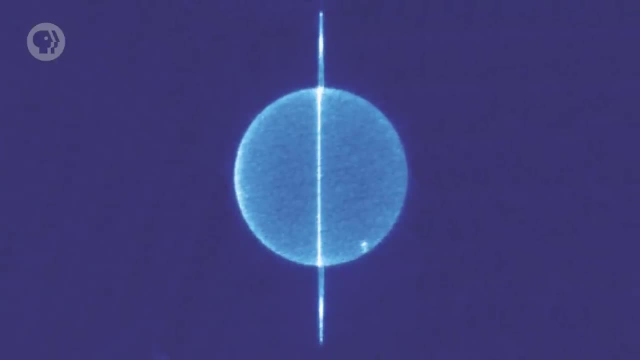 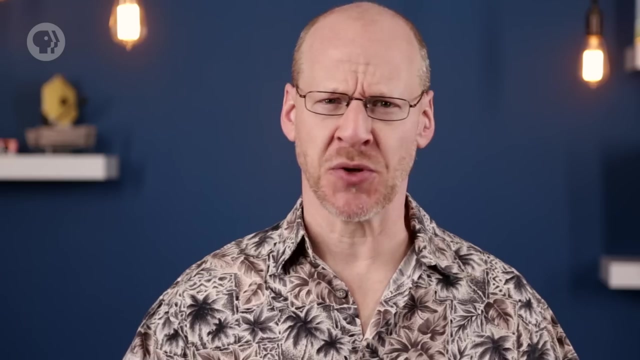 They may have been created by an impact completely shattering a small moon orbiting Uranus, but, as for now, the ring origins are unclear. And then, finally, we have Neptune, the guardian of the solar system's nether regions. Neptune is an ice giant, like Uranus, and has a lot of similarities. 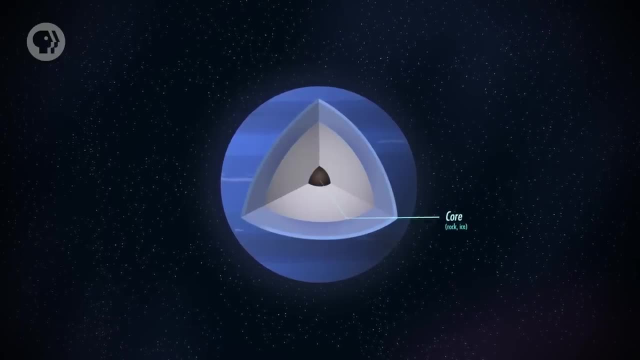 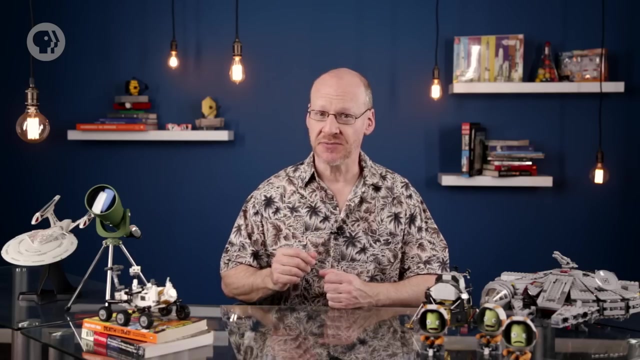 Like its green brother, it probably has a rocky core surrounded by a thick, icy mantle of water, ammonia and methane. Above that is an atmosphere of hydrogen helium and methane. But there are differences too. Neptune is more massive than Uranus: 17 times Earth's mass versus just 14 and a half. 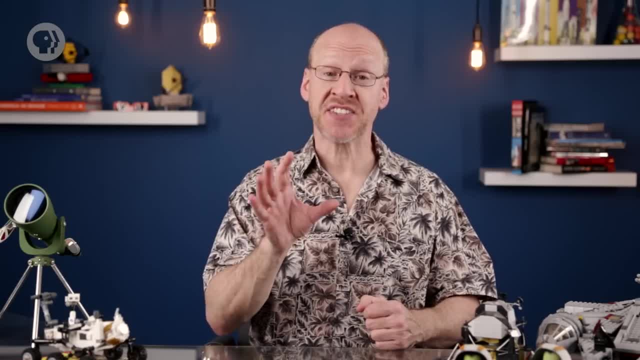 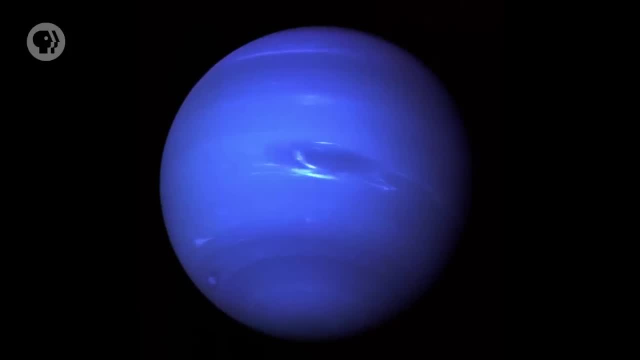 for Uranus. Neptune is slightly smaller than Uranus, which means it's a lot denser. Also, while Uranus is teal, Neptune is a deep, rich azure. I like to call it the other blue planet, the first one being, you know, Earth. 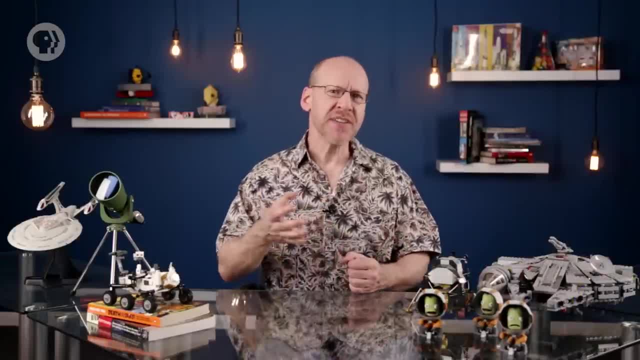 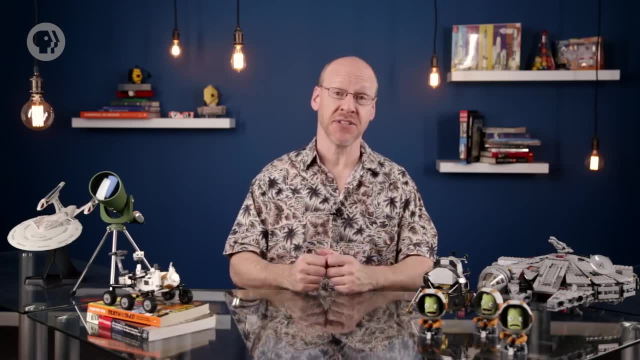 Through a telescope. Neptune's color is quite lovely. It has roughly the same amount of red light-absorbing methane in its atmosphere as Uranus does, so its deeper blue hue is something of a mystery. That may have to do with its active atmosphere. 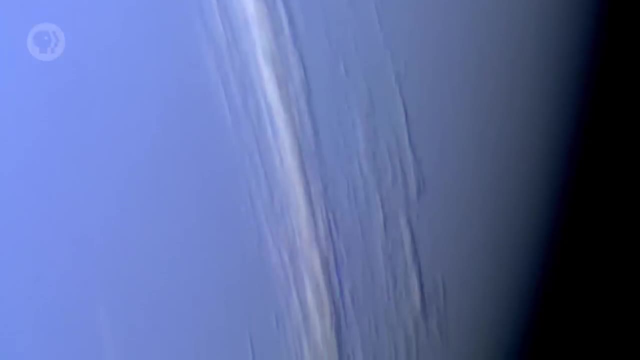 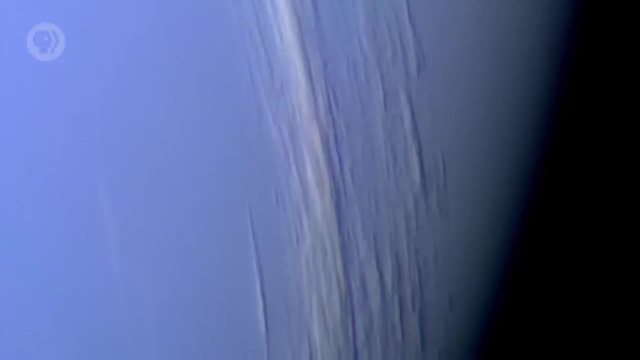 Unlike blander Uranus, Neptune has clouds of methane, ammonia and hydrogen sulfide lying in the skies at different depths, and white streaky clouds were seen during the Voyager 2 flyby in 1989. They looked whipped by wind, and for good reason. 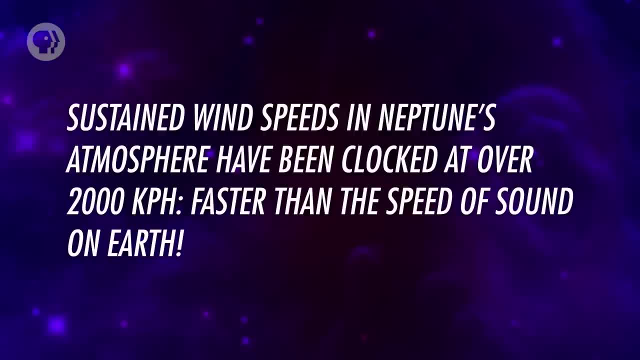 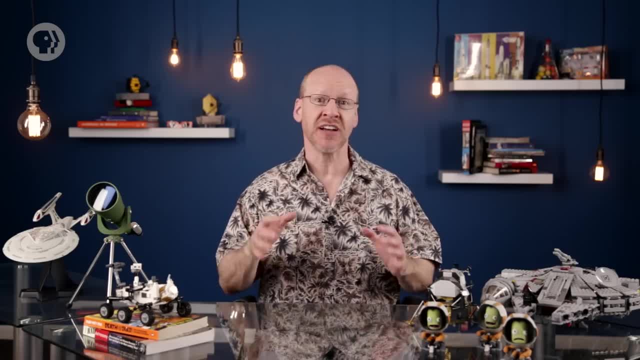 Sustained wind speeds in Neptune's atmosphere have been clocked at over 2,000 kilometers per hour, faster than the speed of sound on Earth. It's thought that the low temperatures in the atmosphere reduce friction, allowing the winds to gather to such amazing speeds. 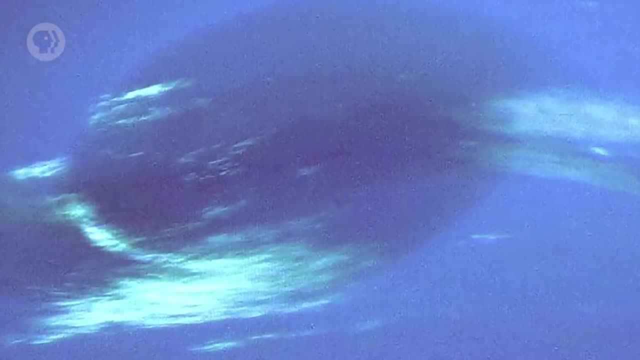 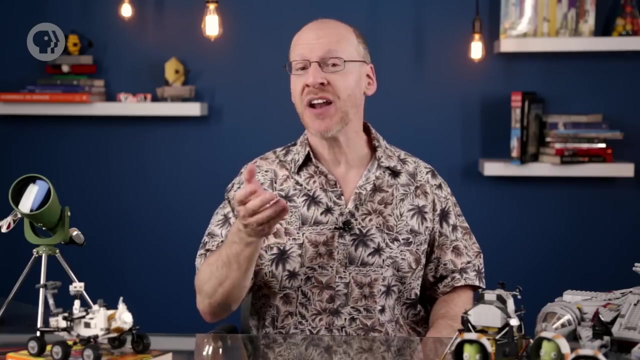 But that's not all. There was a huge storm marring Neptune's face called, for some reason, the Great Dark Spot. A few years later, when Hubble was used to observe the planet, the spot was gone, but others had appeared. 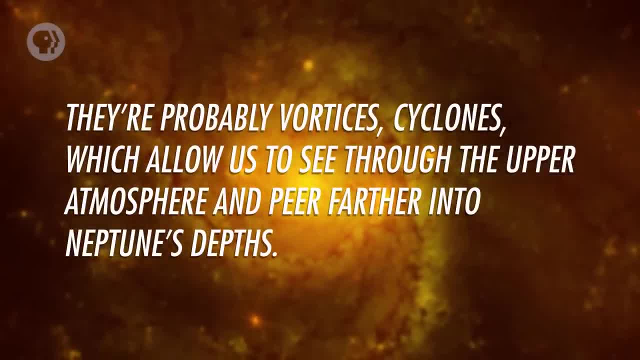 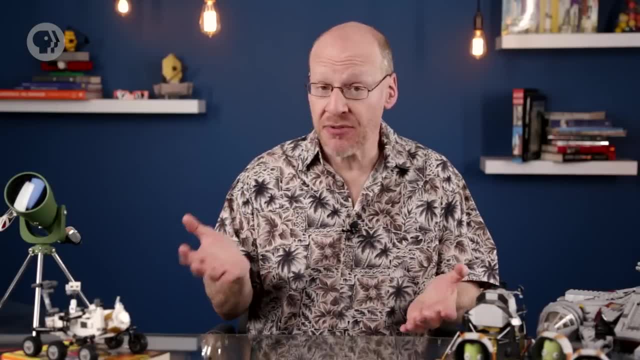 They're probably vortices, cyclones, which allow us to see through the upper atmosphere and peer farther into Neptune's depths. Neptune has a magnetic field and, like Uranus, it's offset from the planet's center. Perhaps that icy mantle is at work, somehow interfering with the generation of the magnetic. fields in both planets. Neptune has rings too, But, shocker, they're weird. There are three main rings, two narrow and one broad. They're clumpy and have bright stretches that make the rings look more like incomplete arcs. 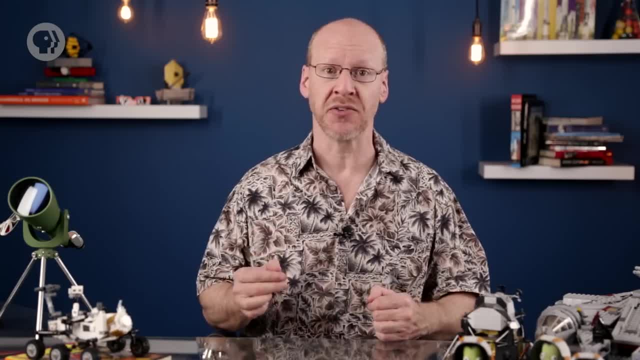 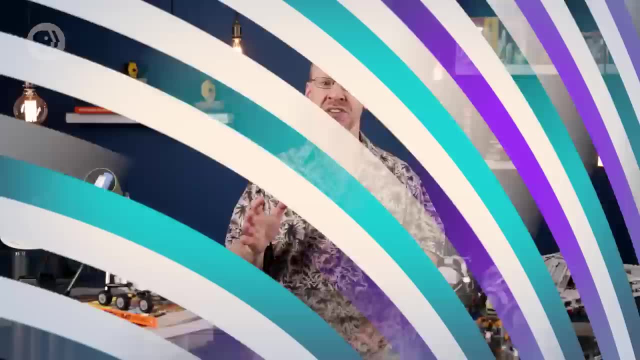 It's possible. those arcs are being constrained by small moonlets near the rings, Speaking of which, Neptune has over a dozen known moons. Most are quite small, but one, Triton, is by far the largest, At 2,700 kilometers across. it's smaller than our own moon, but the rest of them are. 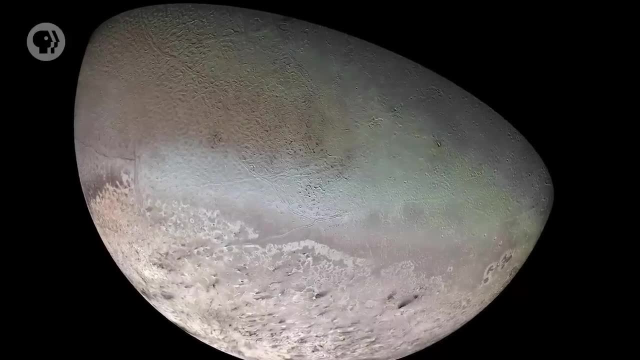 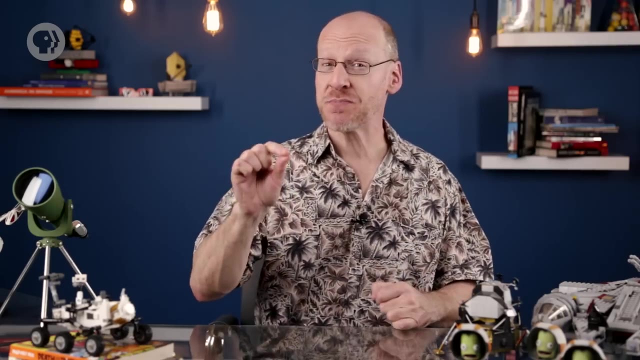 really dinky. Triton orbits around Neptune backwards Retrograde. As we'll learn in a future episode, there's a repository of giant iceballs out past Neptune, so Triton was probably one of those that got too close to Neptune and was captured by its 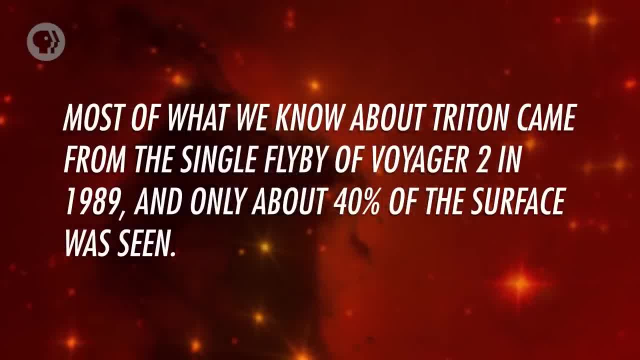 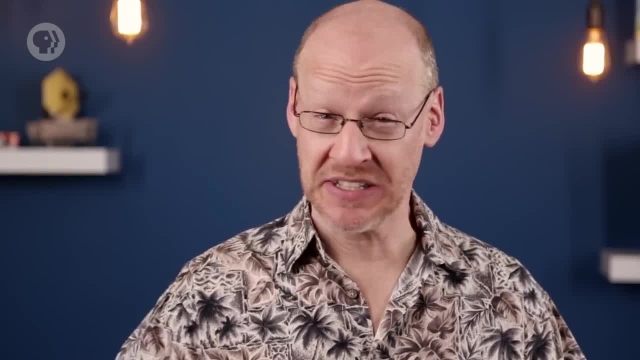 gravity. Most of what we know about Triton came from a single flyby of Voyager 2 in 1989, and only about 40% of the surface was seen. But this quick glimpse revealed a weird little moon. The surface is covered in nitrogen ice, as well as water and carbon dioxide ice. It's really flat and has very few craters, meaning something resurfaces. Something resurfaced it in geologically recent times. Most likely this was from cryovolcanoes, cold volcanism, that is, volcanoes where water. 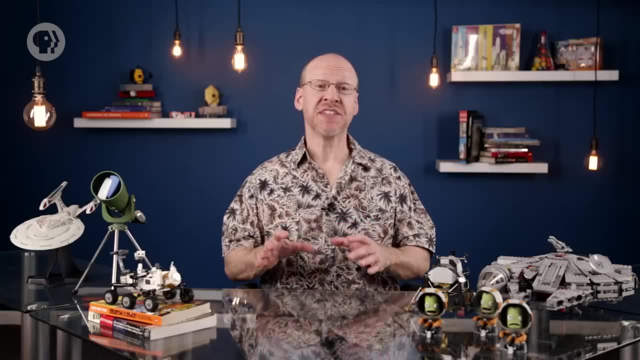 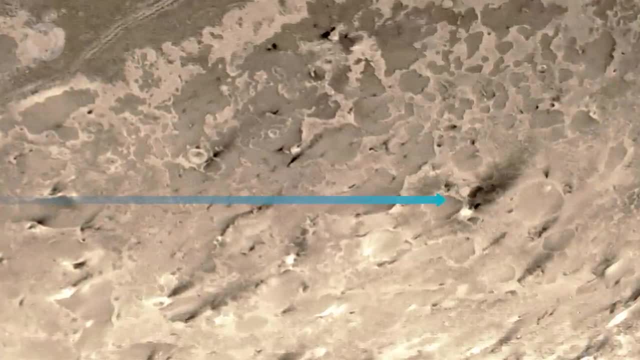 and ammonia take the place of lava there. Also, Triton has been seen to have active geysers of nitrogen erupting from its surface. They're probably due to warming from the Sun, and they make Triton one of the few objects in the solar system seen to be geologically active. 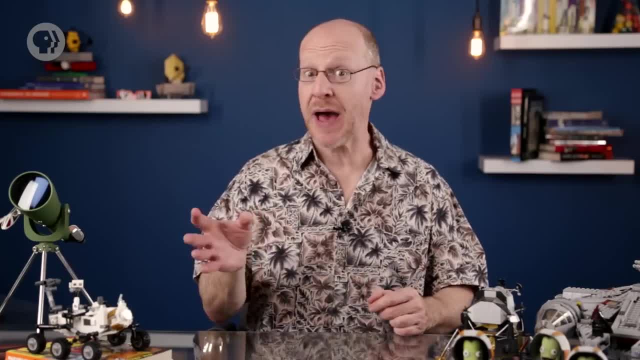 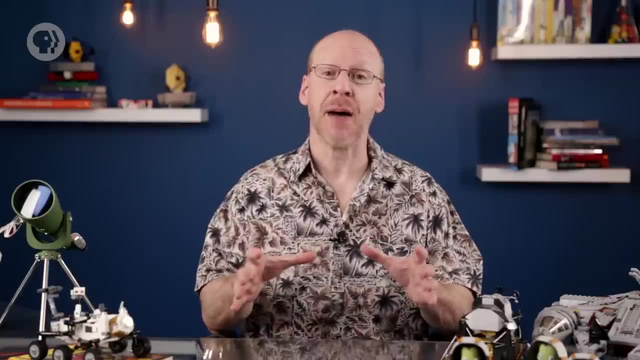 It also has a very thin atmosphere of nitrogen, probably due to evaporation from the surface. After all, this Neptune is special in another way too. Neptune is faint and can only be seen telescopically. It was discovered in 1846, and it wasn't an accident. 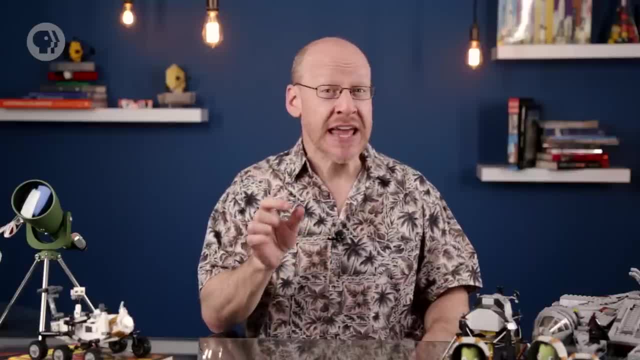 Over the decades, astronomers observed Uranus and found out that it was not an accident. But there's more. They found something weird. It wasn't where it was supposed to be. Over time, its predicted position was off from where it actually was. 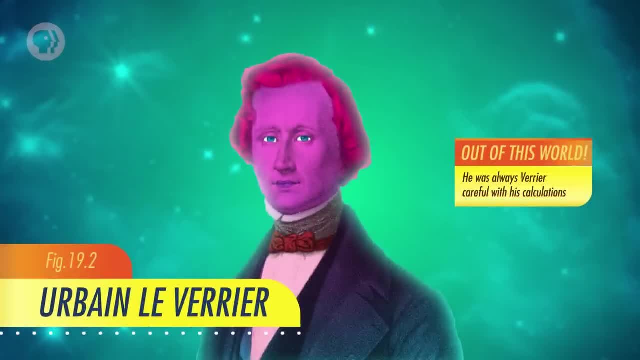 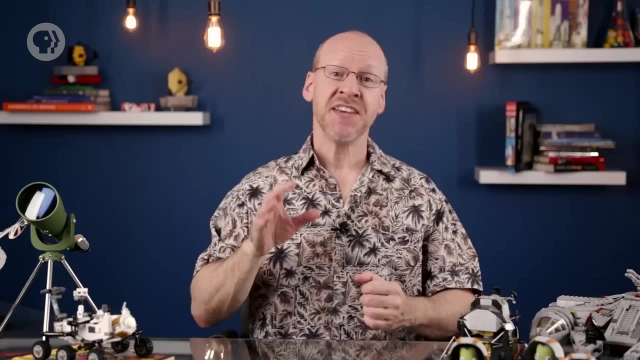 The French mathematician Urbain Le Verrier concluded that this was due to an unseen planet and was able to use the mathematics of orbital mechanics to predict where the new planet would be. He sent a letter with the predicted position to the Berlin Observatory. 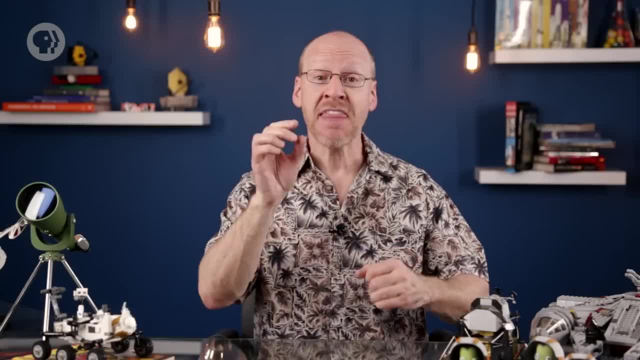 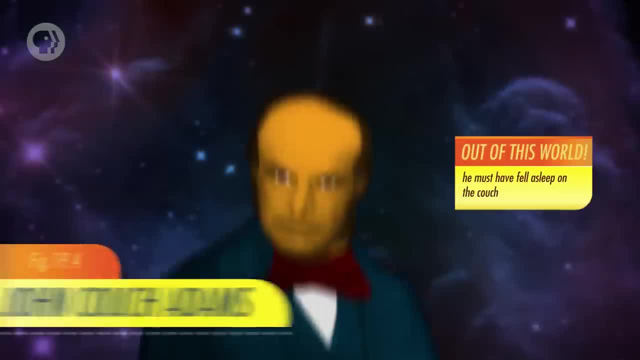 Astronomer Johann Gala read the letter, went right out and found the planet that very night. Neptune was within a degree of the predicted spot. Amazingly, another mathematician, Englishman, John Couch Adams, had also worked on the math and had made a similar prediction.